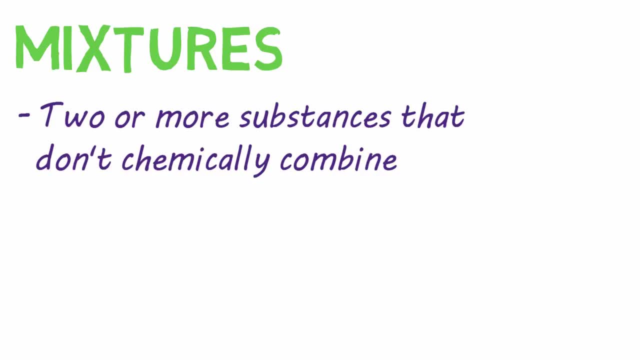 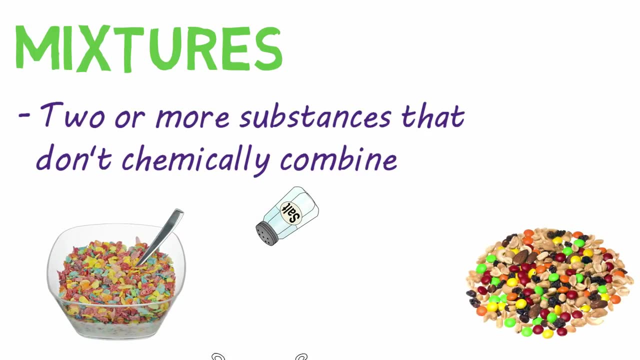 That is, each substance maintains its individual properties. This includes obvious examples like a bowl of cereal or trail mix, but also more subtle examples like salt mixed in water or a soda like Coke. In each case, there are two or more substances mixed which don't chemically combine. 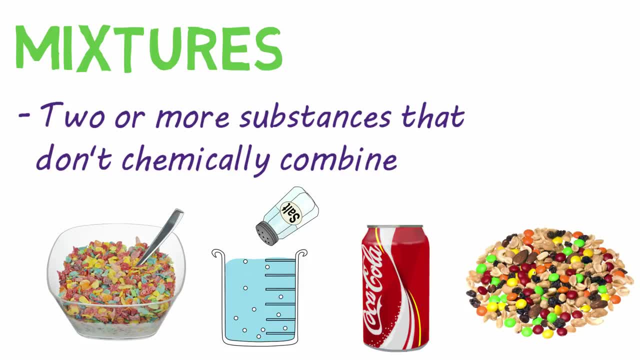 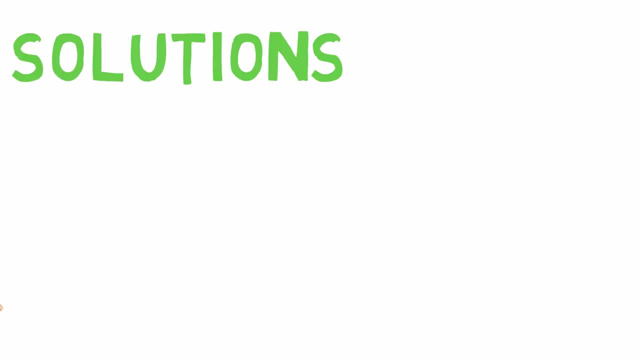 In the soda example, we not only have a mixture of ingredients that make up the liquid, but the carbon dioxide gas mixed in as well. Solutions are a subtle sidestep from mixtures, So the last two mixture examples- salt water and soda- are also solutions. 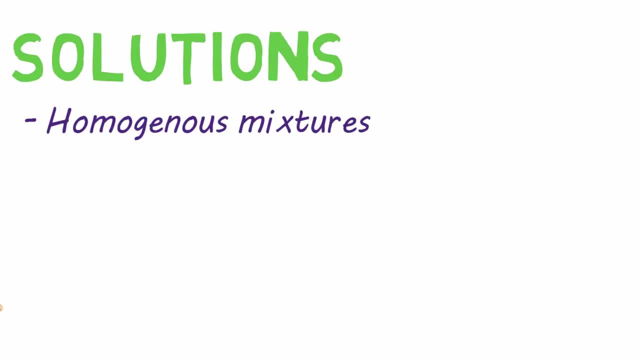 Solutions can also be defined as homogenous mixtures, because there is an even distribution of all the substances. This means that if you took a random sample of any part of the solution, it would have the same ratio of salt to water or carbon dioxide to liquid, for example. 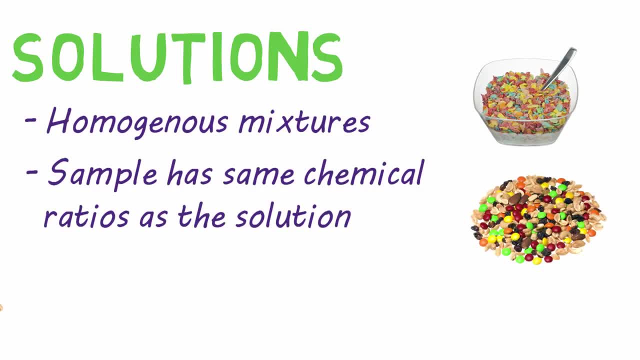 Our first two mixture examples, cereal and trail mix, are not solutions because they are not homogenous. One spoonful of cereal may have more milk than the previous one, or a handful of trail mix may have a higher ratio of peanuts than the entire bag. 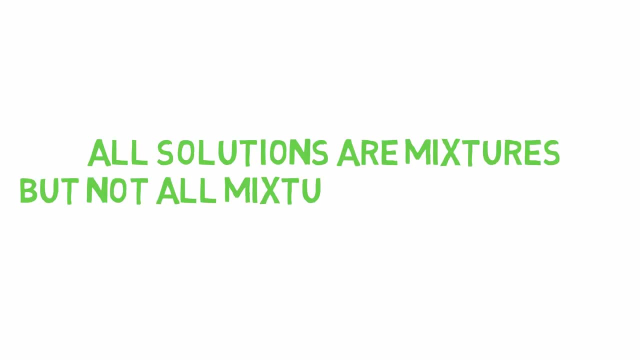 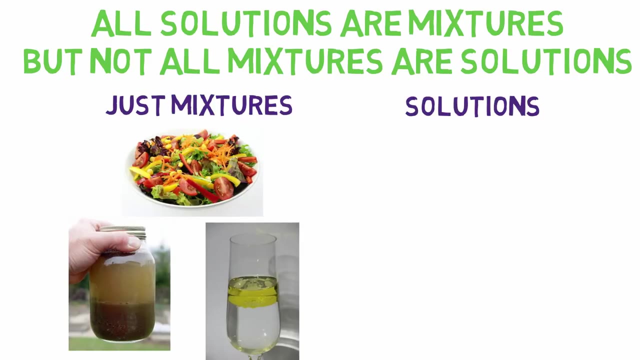 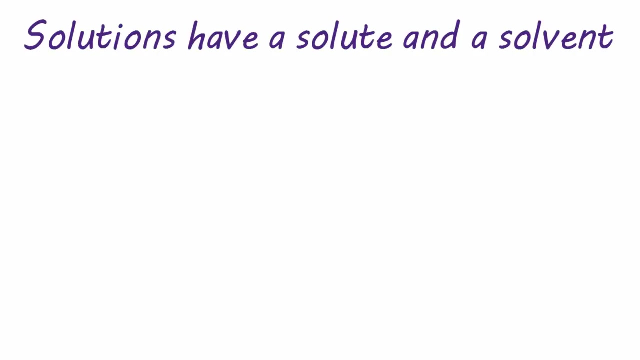 This means that all solutions are mixtures, but not all mixtures are solutions. Here are a few more examples of mixtures and solutions. It's also important to note that solutions have a solute and a solvent. The solute is what is dissolved into the solution. 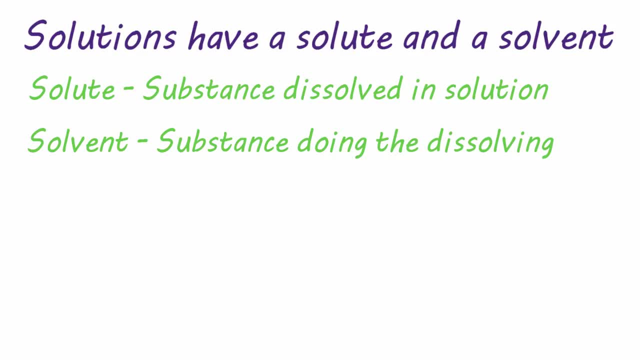 and the solvent is a substance, often a liquid, doing the dissolving. So in our salt water example, salt is the solute being dissolved and water is the solvent doing the dissolving. Hopefully that gives you a good idea of what distinguishes a solution from a mixture. 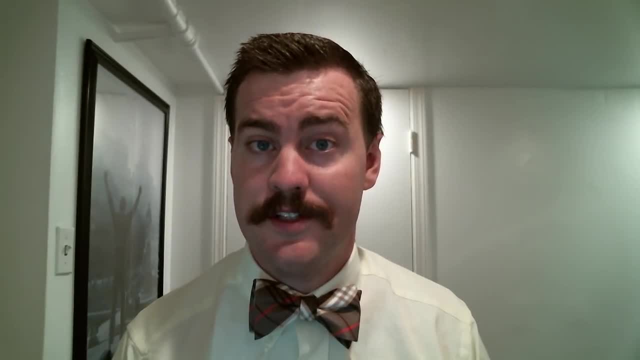 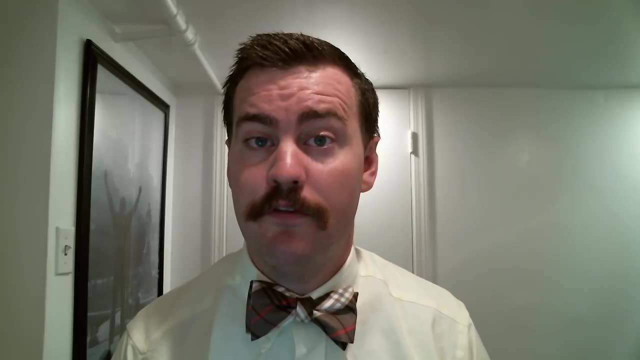 Just remember: a mixture is any combination of two or more substances that don't chemically combine, and a solution is a homogenous mixture, meaning that the ratio of substances is uniform throughout the mixture. One of my favorite mixtures is cookie dough, because, of course, you can make cookies with it. 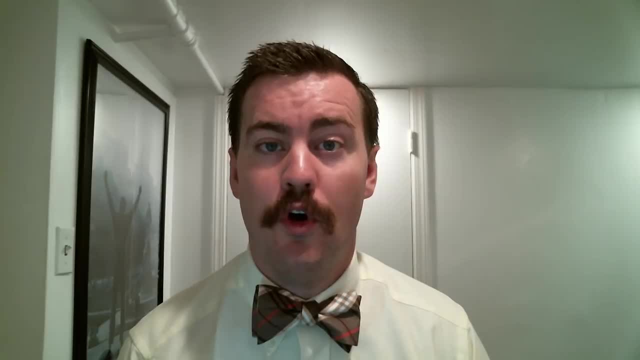 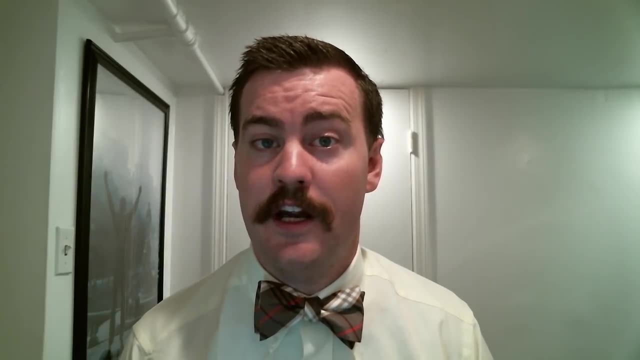 I'm going to be ramping up my video production over the next couple weeks, so be sure to subscribe and catch more of those videos. I should be doing a full biology course over the next year and then getting into some chemistry and physics and other things.